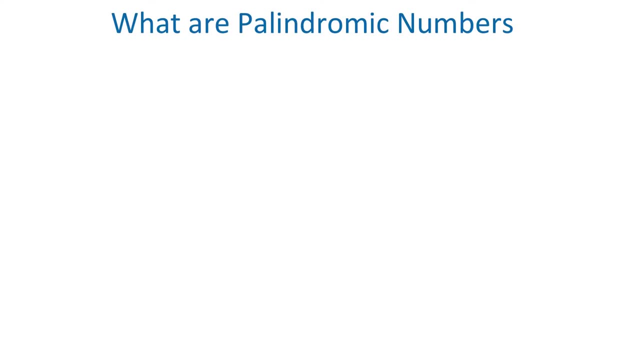 So what are palindromic numbers? These are numbers that stay the same when the digits are reversed. For example, the number 245,542 is a palindromic number. If we read the digits from the left, they are 245,542,. 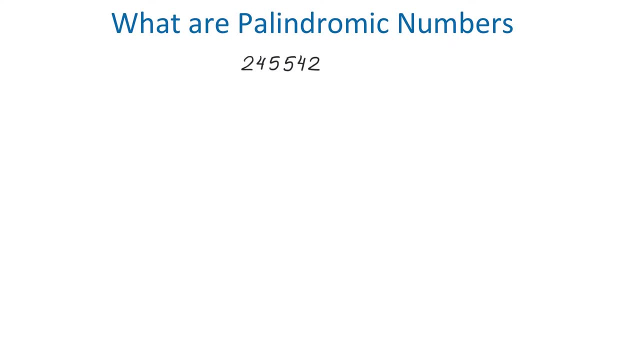 and if we read them from the right, they are also 245,542.. Another example of a palindromic number is 767.. This number also remains the same if the digits are reversed. And do you know that all the one-digit numbers are also palindromes? 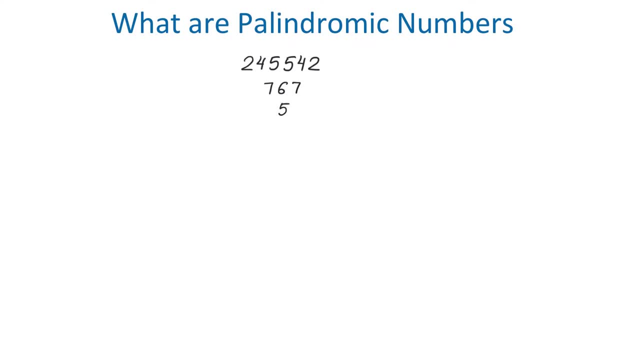 For example, we can say that number 5 is a palindrome. Now I will write for you the list of the first few palindromic numbers. The list starts with 0 and then includes all the one-digit numbers from the left. If we read the digits from the right, they are 245,542,. and if we read 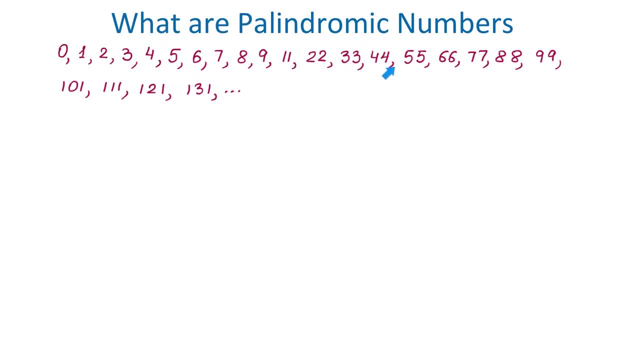 the digits from 1 to 9, then we have 9 two-digit palindromic numbers. then the list continues indefinitely. A recent proof done in mathematics shows that we can take any positive integer and we can write it as a sum of three palindromic numbers. For example, we can write the number 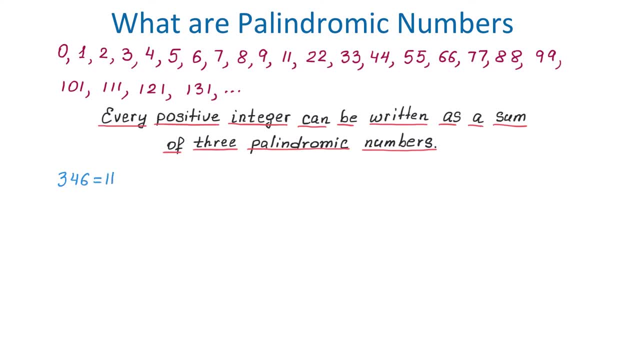 346 as 11 plus 22 plus 346.. As you see, all these three numbers represent palindromes. We can also represent 346 as 343 plus 3 and plus 0. These three numbers also represent palindromes. The number 170 can be. 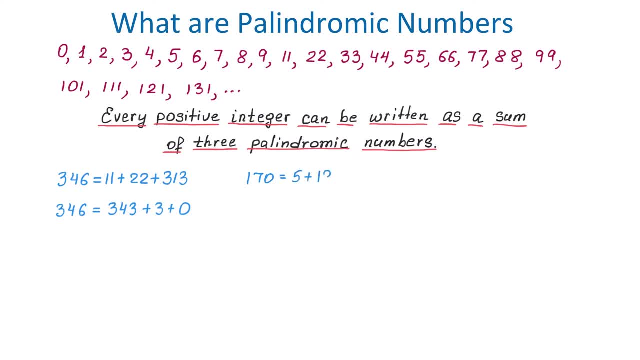 represented as 5 plus 121 plus 3.. Or it could be represented as 66 plus 101 plus 3, or 161 plus 9 plus 0.. As you see, each of these numbers can be represented by a different group of palindromic numbers. 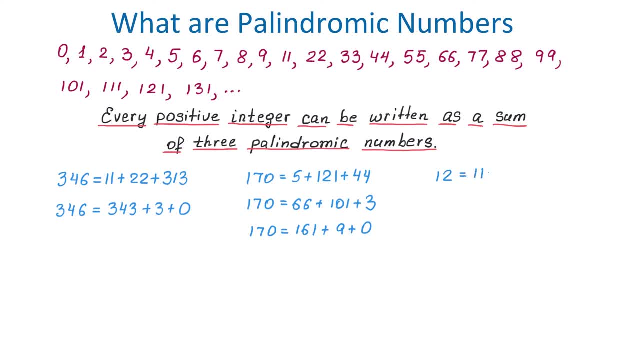 Number 12 can be represented as 11 plus 3.. Or it could be represented as 7 plus 7 plus 1 plus 0.. Or it could be represented as 5 plus 5 plus 2.. And these are just two ways we can represent number 12 using palindromic numbers. 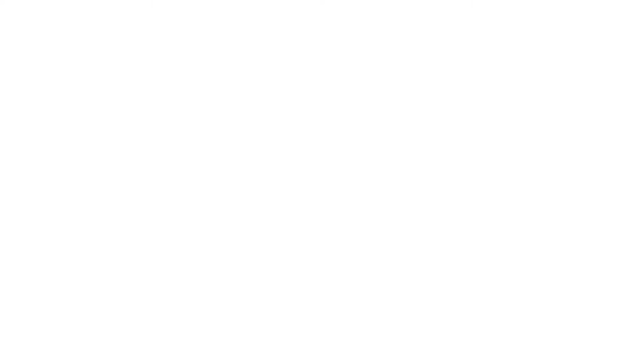 Another interesting thing about palindromes is that we can take a number, for example number 125, then we reverse the digits to get 521.. And now, if we add these two numbers, we will get a palindrome, and this will be 646.. 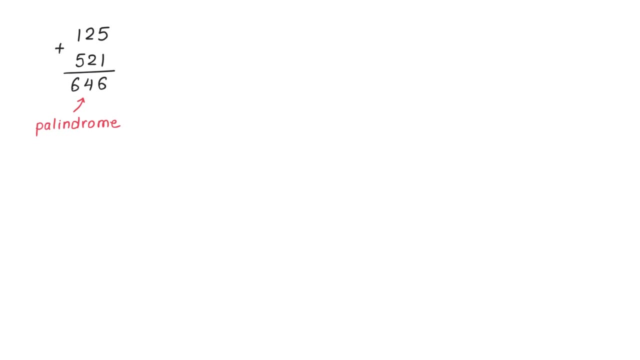 This process is called the reverse and add process. Now I will try another number, for example 129.. If we reverse it, we get 921.. Now let's add the digits From the right. we will have 0. Then 5.. 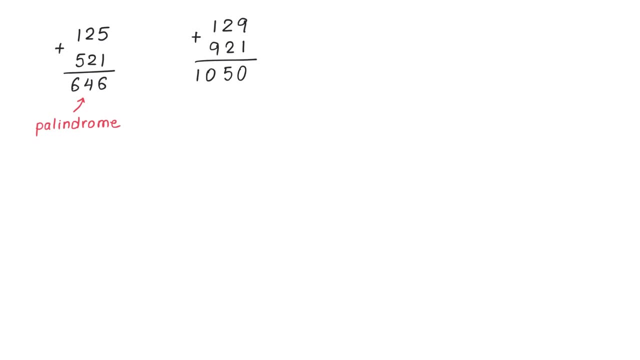 And 1 plus 9.. 8. Is 10.. As you see, 1050 is not a palindrome. but let's repeat the process by reversing 1050.. So we have 1050.. And if we reverse it, we get 0501.. 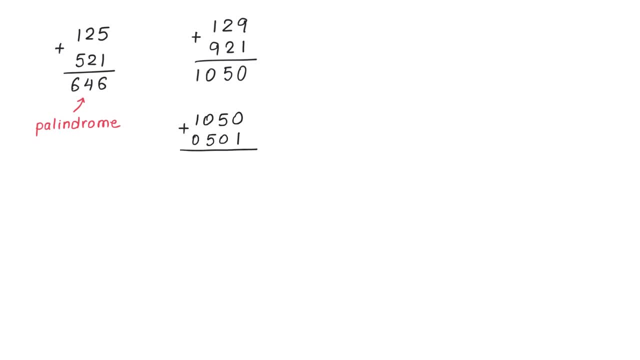 And now let's add these two numbers, The result will be 1551.. So in this example, after two steps, We got a palindrome. Now let's see one more example. I will choose a random number, for example 59.. 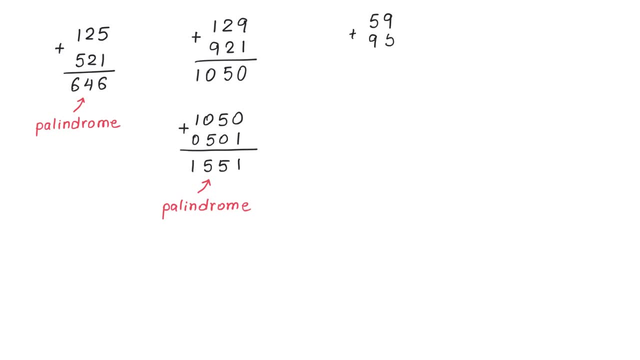 And now, if we reverse it, we will have 95.. The result will be 154.. So far this sum did not produce a palindrome. therefore, let's take 154 and add 451.. The result here was 154.. And now let's add 451. 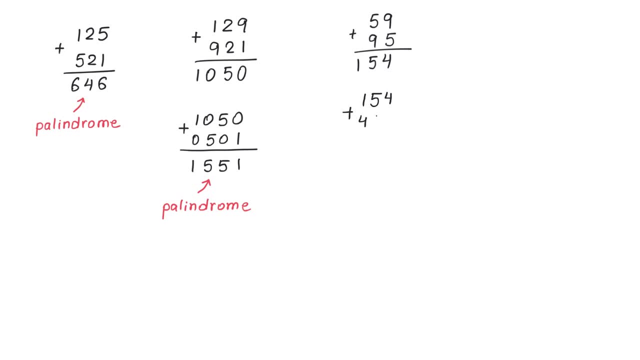 So in this example, after two steps we got a palindrome. And now let's take 154 and add 451.. The result will be 154.. So in this example, after two steps we will have 154.. The result here was 154. 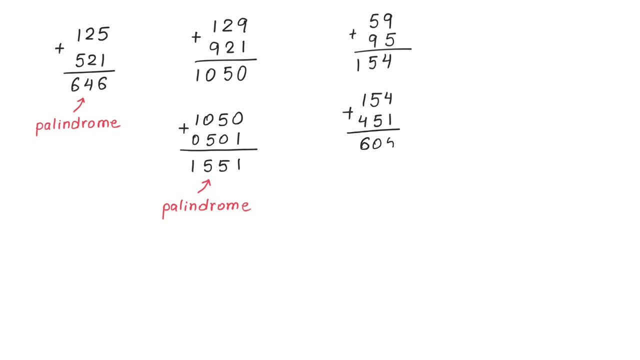 And now let's add 451.. The result here will be 605.. So we still don't have a palindrome. therefore, let's continue with the same steps. We will take 605.. And we will reverse it and get 506.. And now let's add: